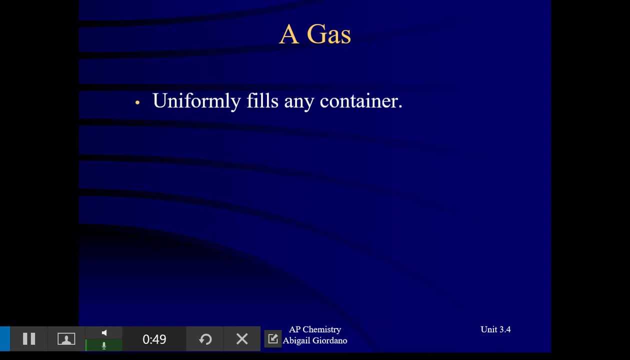 characteristics. So when a gas is in a closed container, it will fill the volume of that container. Okay, so gases have very variable volume. Okay, they can expand, they can contract. If you mix more than one gas together, multiple gases- they will mix spontaneously. It's not like 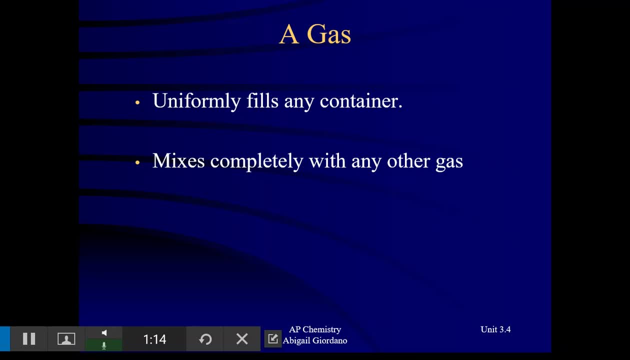 you have to stir them with a stick. They mix naturally, And gases exert pressure on whatever they are around, And we're going to talk a little bit specifically about what that means. So let's get started. What is pressure? How do we understand it? So pressure is defined as a force exerted over some. 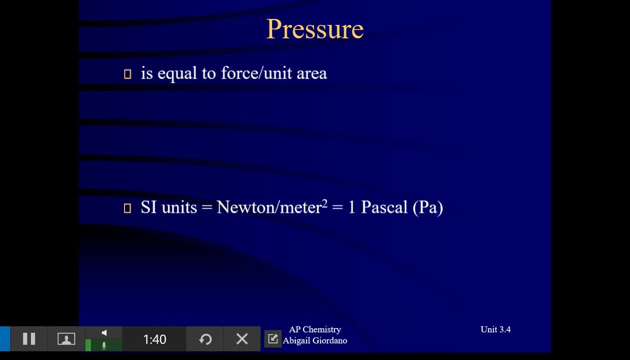 unit some area. Okay, force per unit area. And if we were in a physics class, you talk about forces in units of newtons. A newton per meter squared is a unit of pressure called a pascal. Now, we will not use units of pascals very often. More often, we will be using 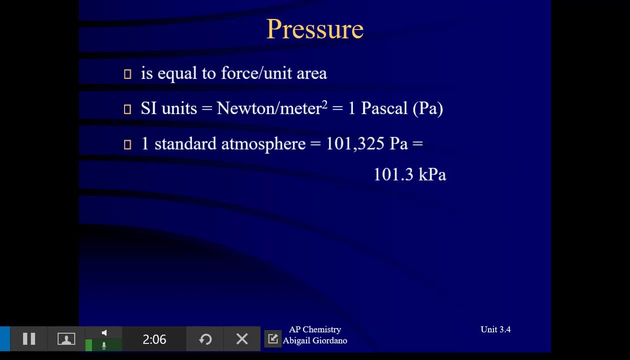 units of pressure, atmospheres and kilopascals, All right, but let's come back to that whole force per unit area thing. Okay, I want you all to have an understanding of what pressure is And you can kind of visualize it. All right, so if you have a container with a sample, 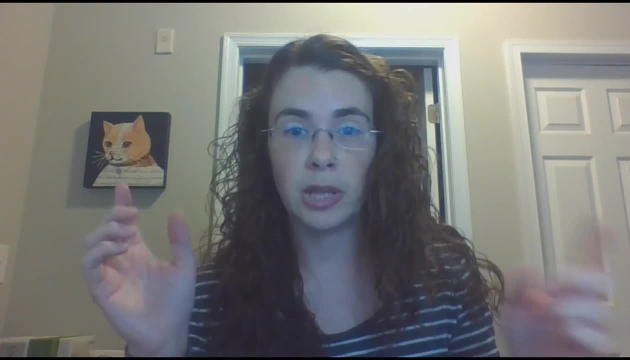 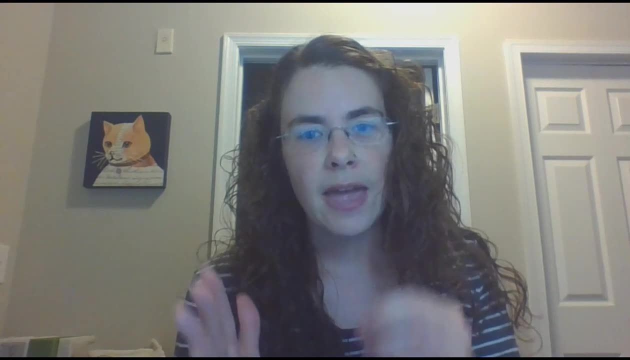 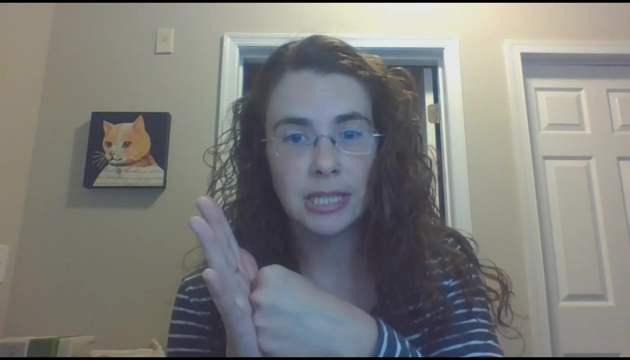 of gas in it. imagine what those particles are doing. They're moving around and they're super fast and they're bouncing off the walls and they're bouncing off each other. Every time one of those gas particles strikes the side of its container, it's exerting a force over that area. 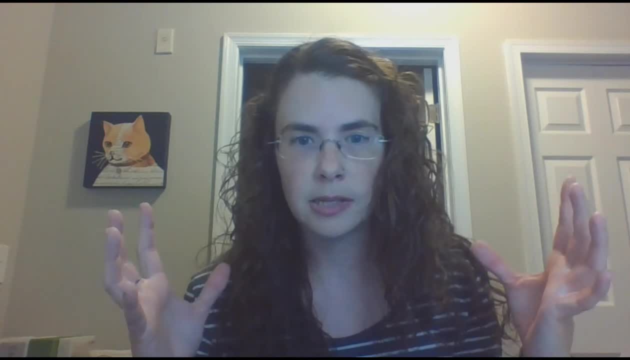 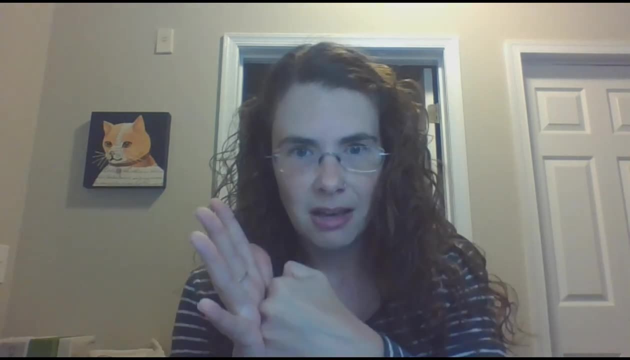 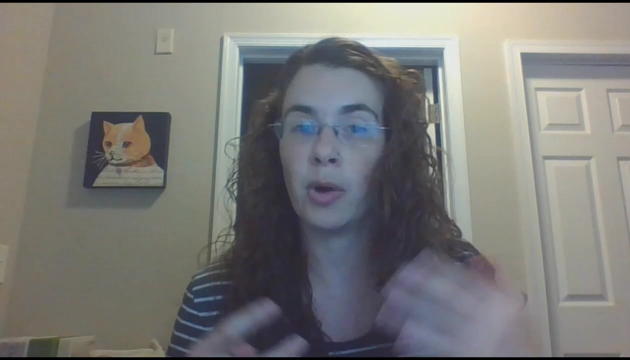 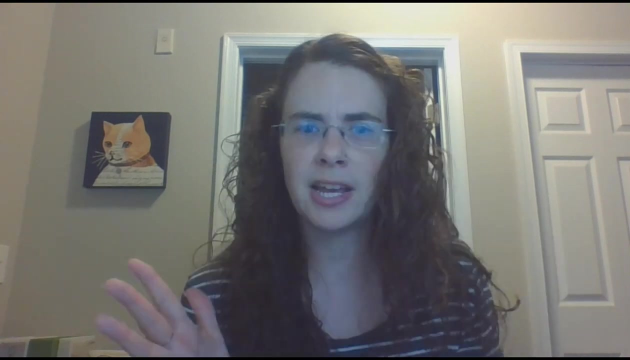 So here's how I want you to sort of visualize pressure. Pressure is like the number of hits on the side of the container: The more hits there are, the higher the pressure is If, whatever our situation, we're causing there to be fewer hits on the side of the container. 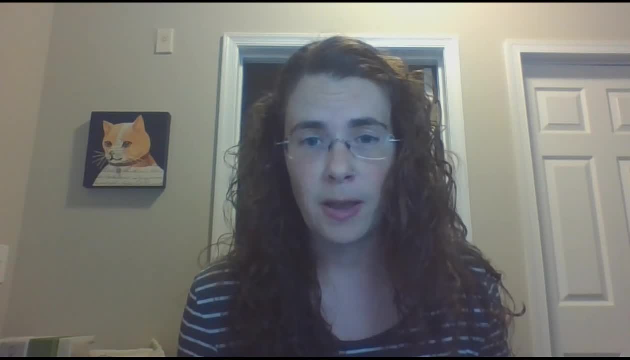 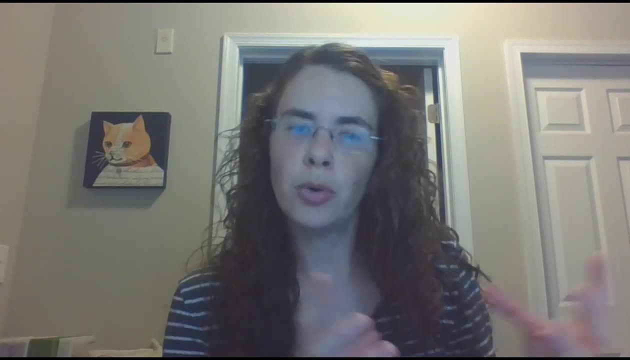 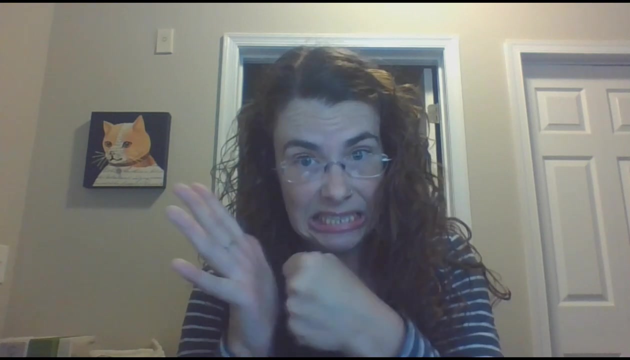 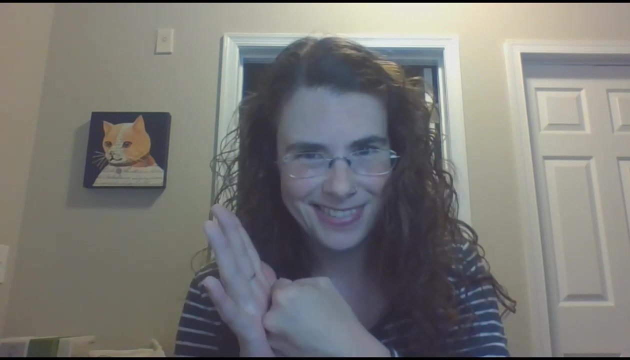 then the pressure must be going down, Okay. so whenever we make a change to a sample of gas, I want you to ask yourself: is what we're doing causing there to be more hits, more frequent collisions on the side of the container, Okay, or is what we're doing causing there to be fewer collisions, Okay? 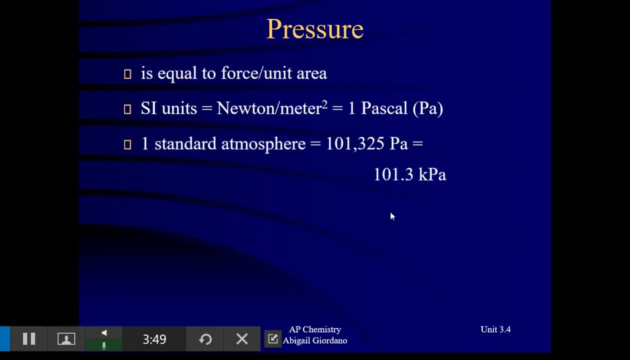 the more collisions, the higher the pressure. Okay, a couple of conversion factors that you should probably know. These are on your equation sheet so you don't have to memorize them. Okay, one atmosphere is equal to a unit called. we see units of millimeters of mercury and torr. 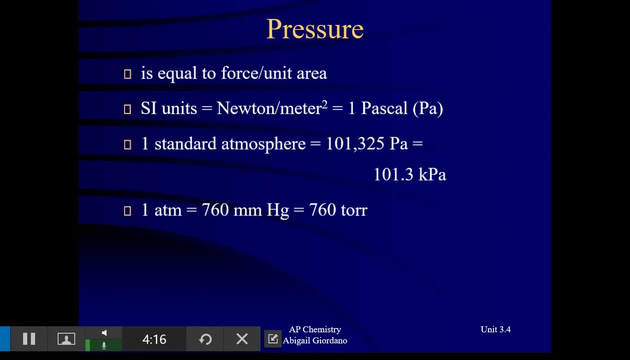 One atmosphere is equal to 760 torr. The units of torr and millimeters of mercury are interchangeable. That unit of millimeters of mercury comes from a barometer, which is just a tool used to measure atmospheric pressure. So again, I want you to visualize the concept of pressure as hits on the side of the container. 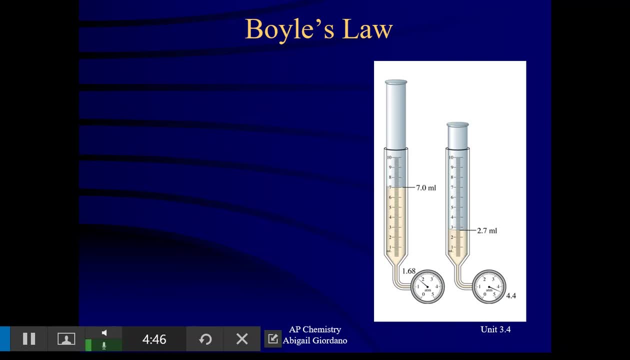 So let's review some of the basic gas laws. This was the first one that you learned back in Chem 1, Boyle's Law, and it links pressure and volume and they are related inversely. Okay, if, like in this picture, we have a sample of 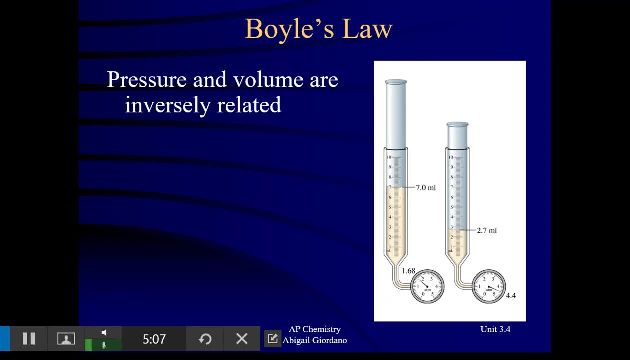 a gas in a syringe and, if you'll notice from the picture on the left to the picture on the right, we have decreased the volume. And look at the pressure gauges: We've decreased the volume and the pressure has gone up. That's an inverse relationship. 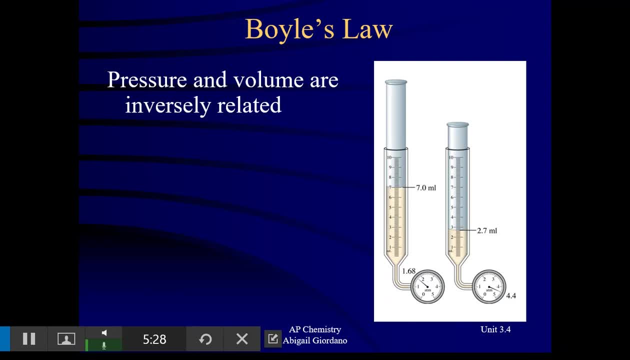 Okay, and it is proportional. If I had cut the volume exactly in half, the pressure would have been exactly doubled. Okay, now, this relationship is only true if temperature is held constant. If you're changing temperature, then we have to use a different relationship. Okay, but this is Boil's law. 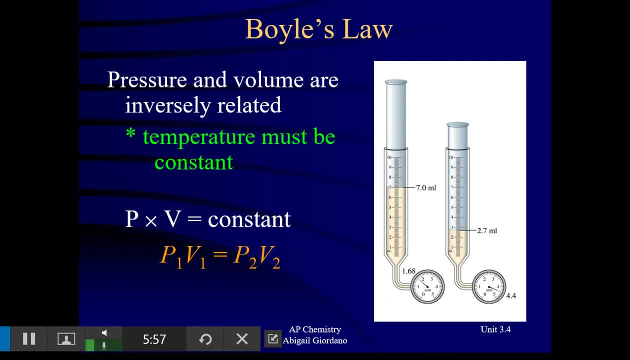 P1v1 equals P2v2. the initial pressure and volume are equal to the new pressure and the new times, the new volume. okay, Units for this equation do not matter, as long as the units are the same on the left and right of the equation or the equal sign. 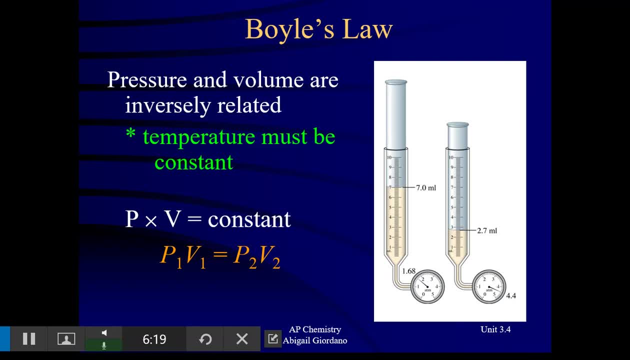 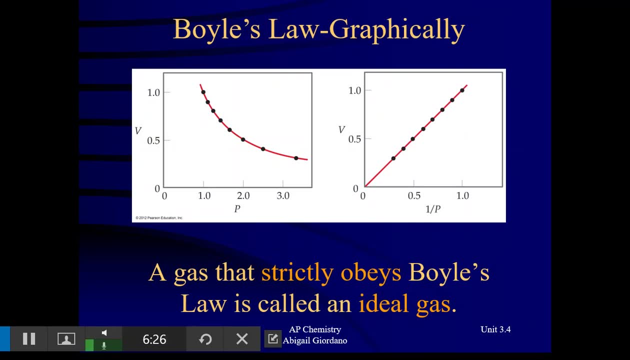 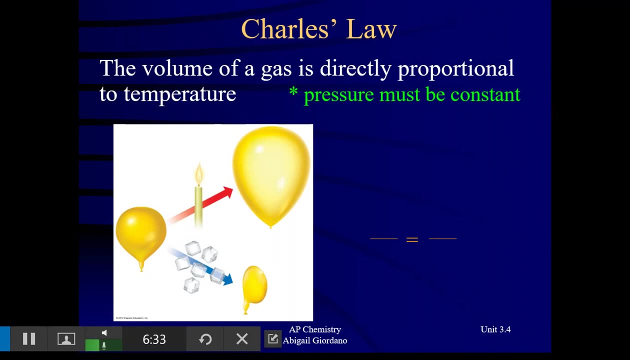 So same unit of pressure on both sides, same unit of volume on both sides. okay, And that's Boyle's law. graphically, Charles' law is our next one. okay, Which relates temperature and volume. okay, And this time it is not an inverse. 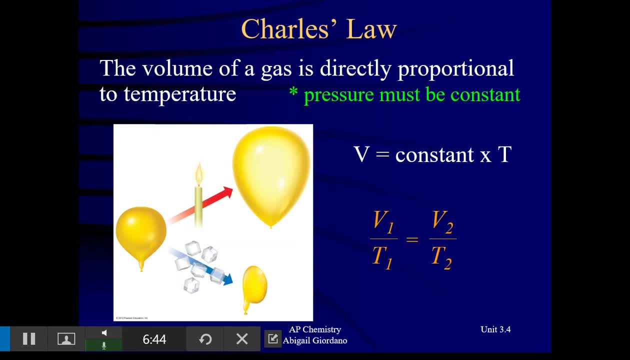 relationship. it's a direct relationship. If you raise the temperature, you will also increase the volume. okay, And this is something that you may have noticed, if you you know, let's say, you buy a balloon in a nice warm store in the 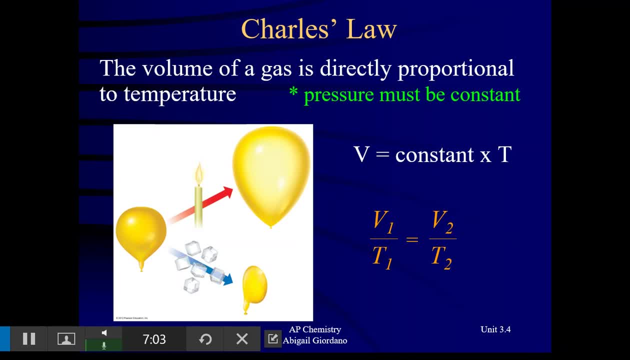 middle of winter and then you take that balloon out to your car in the parking lot and it's really cold outside. Temperature goes down. you'll notice that the balloon goes down. and then you take that balloon out to your car in the parking lot and it's really cold outside. Temperature goes down. you'll notice that the balloon. 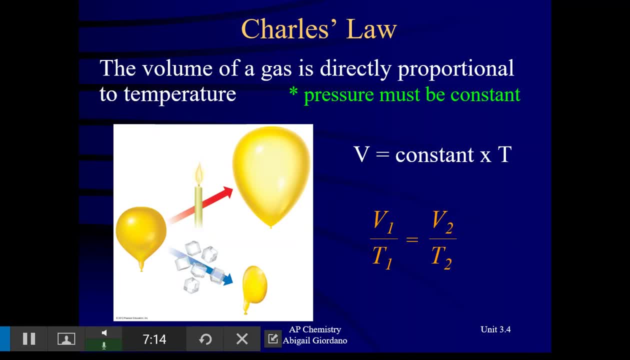 shrinks a little bit. okay, It's a direct relationship. Now, of course, again, this will only hold true if pressure is kept constant. alright, Something that I want to remind you about when you're using these gas law equations anytime you plug. 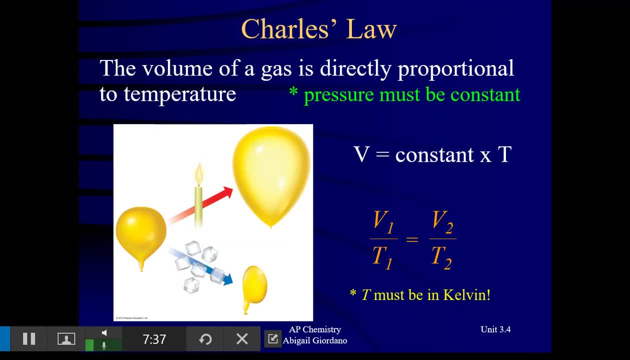 in temperature. it must, must, must be in units of Kelvin. Most of the time, guys, you're going to be given temperatures in Celsius. You need to add 273 to get it into Kelvin and then plug it into your equation. Okay. 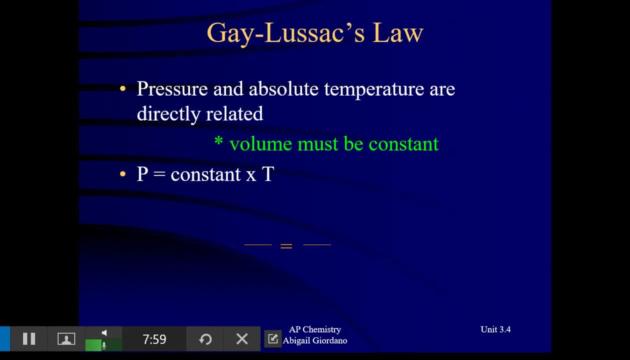 There's Charles' law. graphically, Here's our last one, Gay-Lussac's law, which relates pressure and temperature. okay, Another direct relationship. If you raise the temperature, you will also raise the pressure Again. temperature needs to be in kelvin and. 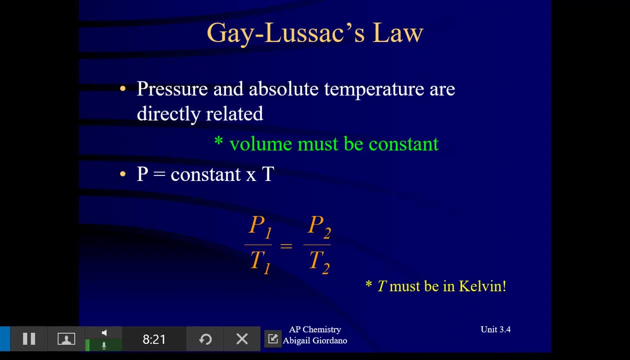 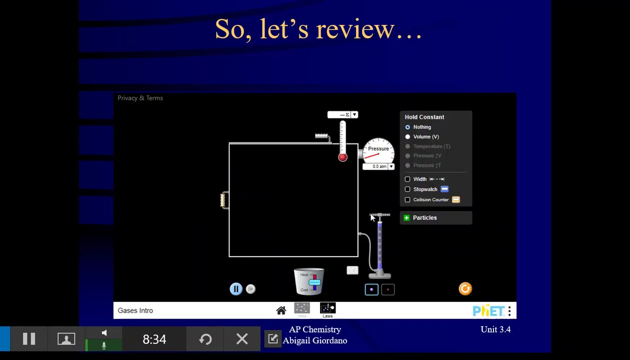 this relationship here is going to hold true only if volume is constant, And we'll talk about what happens if it's not, and what if you're changing all three, We'll get to that, Okay. so I'm going to bring up this little demonstration here. 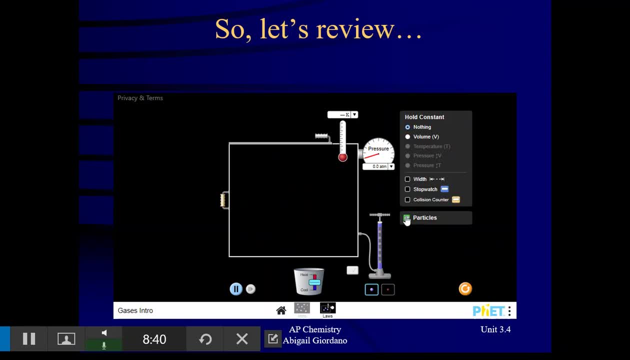 all right, and I'm going to put in some gas into this container. That looks like a good amount, And what I'm going to do is I'm going to make some changes here, all right, and I want you guys to sort of predict what's going to happen. Okay, so let's review. 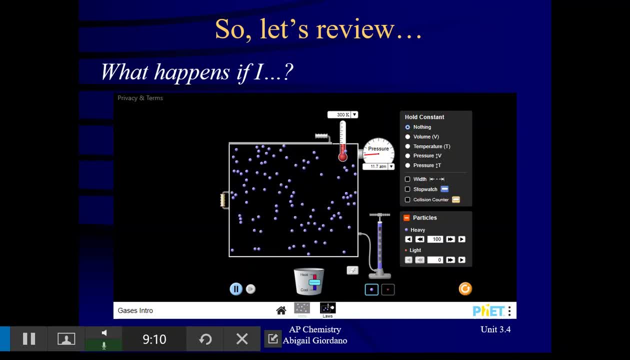 Boyle's Law. Okay, if you'll remember, Boyle's Law held true as long as the temperature was held constant. so I'm going to select that, And what I'm going to do is I'm going to change the volume of this container. okay, and I want you guys to watch this pressure gauge here. all right? 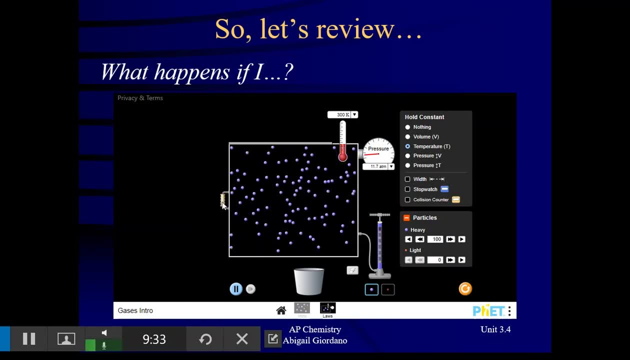 So we're holding temperature constant and I am going to shrink the volume down. so watch, right Now, the pressure is at about 11.7.. Watch what happens. Okay, I reduced the volume by approximately half and the pressure was approximately doubled. Guys, that should make sense to you. I've created less space for these particles to move around. Remember what we said about pressure When I shrunk the volume down. are there going to be more collisions on the side of the container or less? Definitely more. So the pressure goes up. 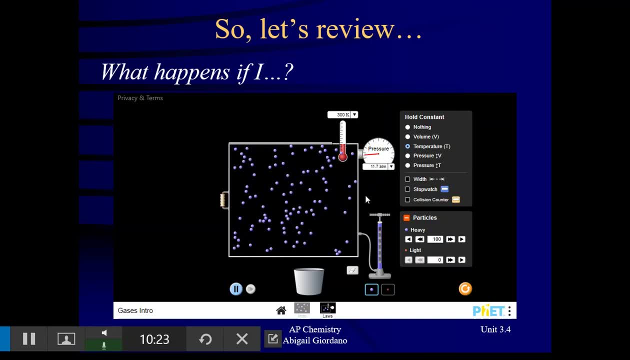 All right, I'm going to put it back. Okay, now let's talk Charles' Law. This time I'm going to keep pressure constant, okay, and I'm going to to increase the heat. okay, I'm gonna raise the temperature. 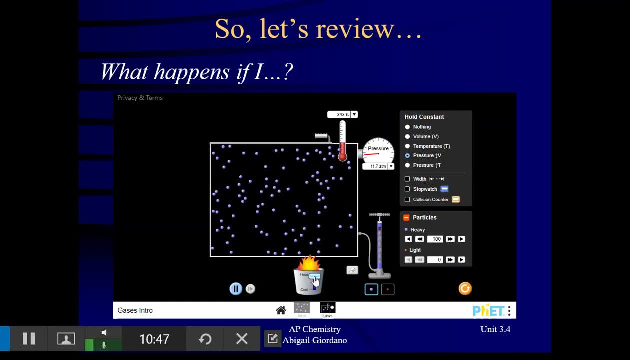 and let's see what happens here. Ooh, look what's happening to the volume. okay, There's Charles' Law right there. If you raise the temperature of a sample of gas, you're giving those particles more energy and they literally are pushing the sides. 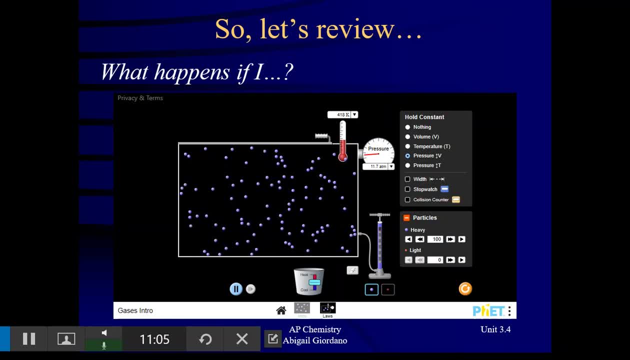 of the container out. okay, Let me move this guy back. Let's test the last one. Okay, I'm gonna keep volume constant this time. So the container is rigid now It can't change its volume. I'm gonna increase the temperature. 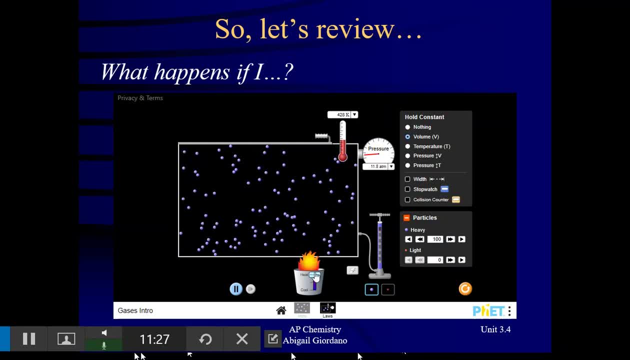 You guys watch what happens to the pressure gauge. watch I'm heating up these gas particles, I'm giving them more energy, and look at what they're doing. They're moving faster, They're making more collisions, So the pressure's going up. 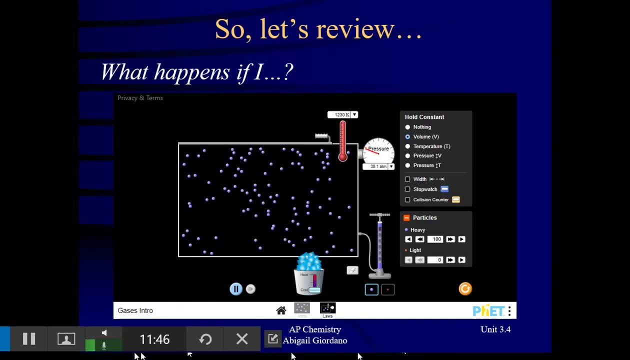 I could go the other way if I want. I could cool this gas down, okay, And it's causing the pressure to drop. Okay, now let's see, I'm gonna hold the volume constant and I wanna show you one last thing. 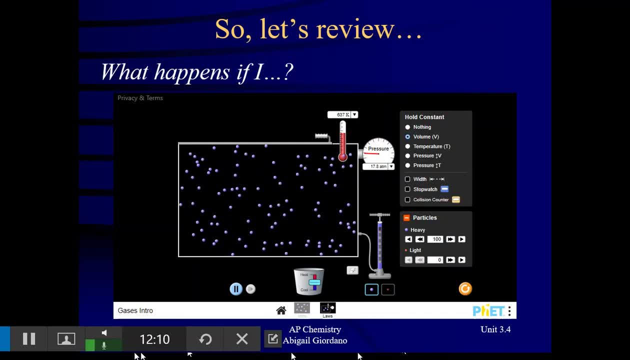 I want you to make a prediction of what might happen if I increase the number of particles in there. What if I inject more gas? There's more moles of gas. The volume's not gonna change. I'm keeping the volume constant. What do you think is gonna happen to the pressure? 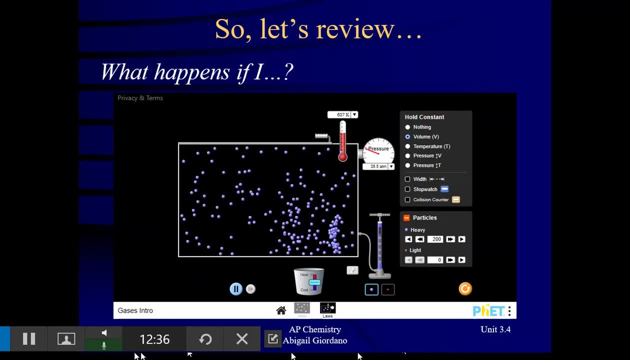 Watch. I've just injected more moles of gas in there and what happened to the pressure? It went up. There's more hits on the side of the container. Okay, so moles of the gas and pressure are also directly related. all right, 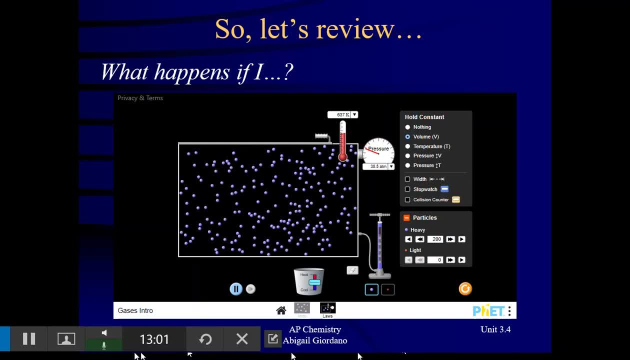 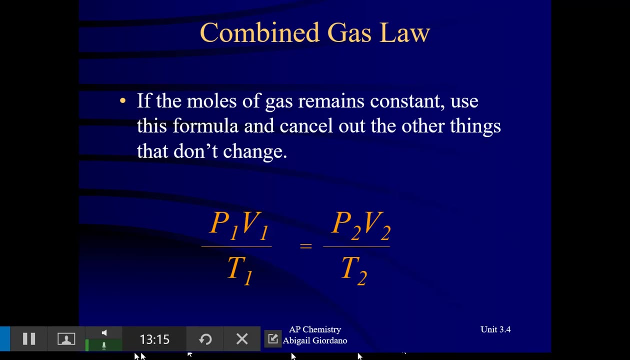 So I wanted to use this visualization so that you could. I don't want you to memorize these relationships, I want you to be able to visualize them And understand them. Okay now, if all three factors- temperature, volume and pressure- are all changing, 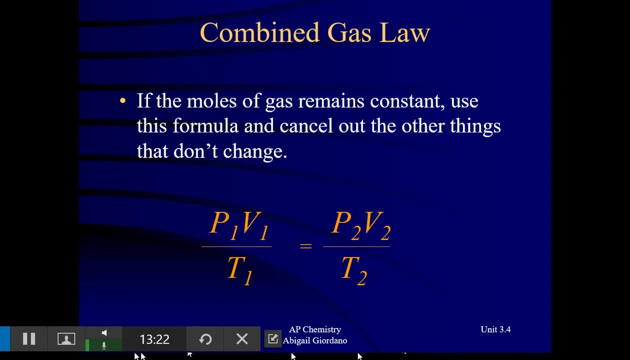 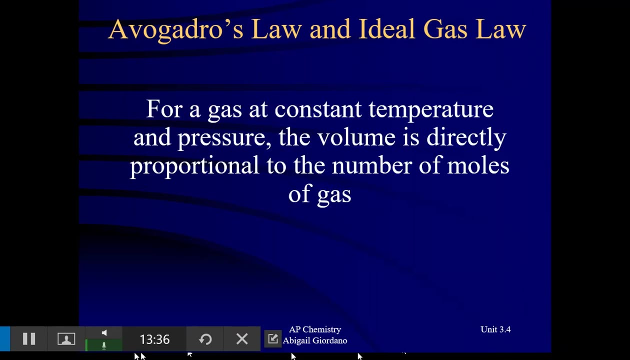 then we use what's called the combined gas law. okay, You probably won't have to use this one very often. It doesn't come up much on the AP exam, but there it is if you want it ever to use it. All right now. we just talked about 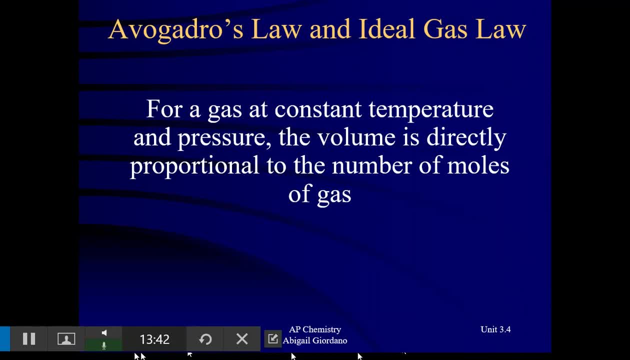 this was the last little demo that I showed you that moles are directly proportional. okay, to pressure when I keep the volume constant, But what if I keep the pressure constant? Then volume is directly proportional. All of these relationships, ladies and gentlemen. 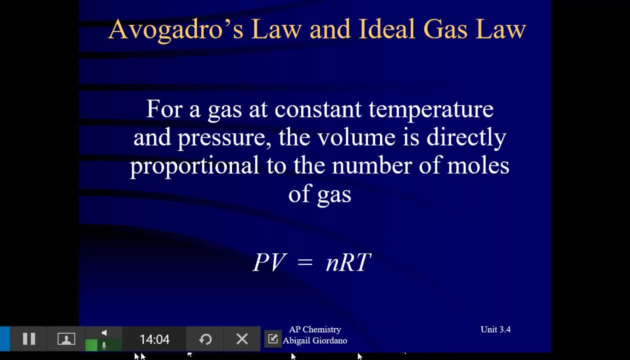 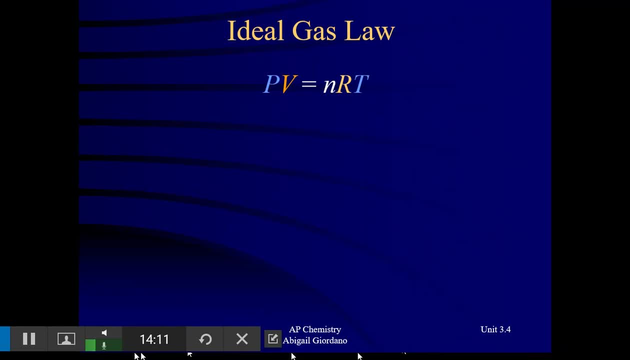 are tied together In the ideal gas law. okay, So let's review that. all right, You learned this in Chem 1, but let's review what each variable represents. okay, P is pressure. of course It can be in units of atmospheres, torr kilopascals. 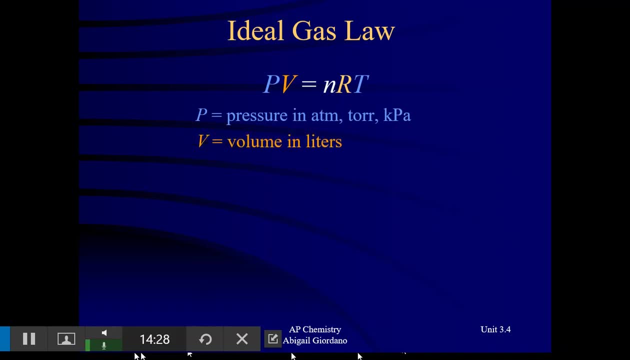 Any of those are acceptable. V is volume. You don't get a choice here for the units. Volume must be in liters. ladies and gentlemen, If you plug in milliliters you're gonna get the wrong answer, okay. N is moles of the gas. 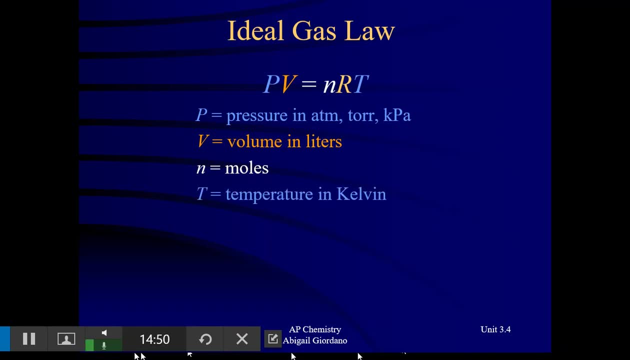 I'll come back to R in just a minute. T is temperature. Don't forget to put it in Kelvin. R is something called the ideal gas constant And, ladies and gentlemen, it has multiple possible values. You do not have to memorize these. 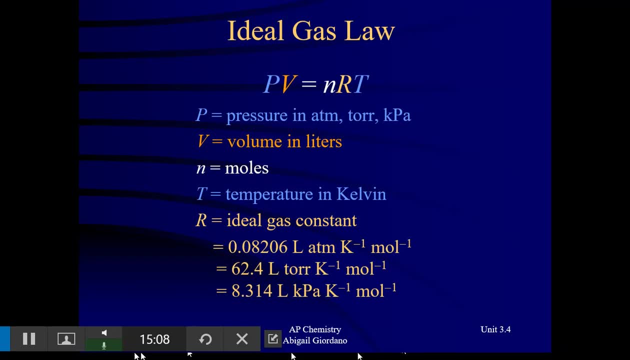 They are on your equation sheet. Look at the different values for the constant. Look at the units. What's the only thing that is different? The units of pressure. all right, So if I am doing a problem where the pressure is given to me, 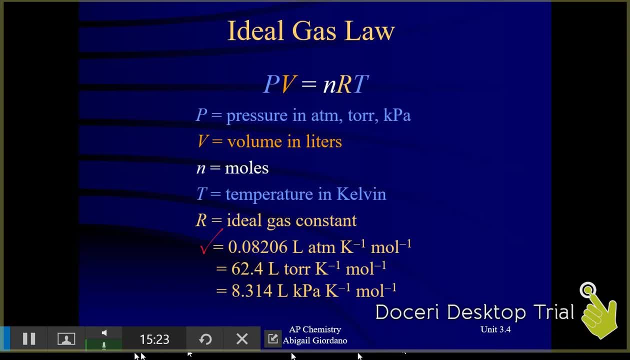 in units of atmospheres, then I'm gonna use that one, that first possible value for R, because it's the one that has units of atmospheres in it. If my pressure is in torr, then I'm gonna use this one. 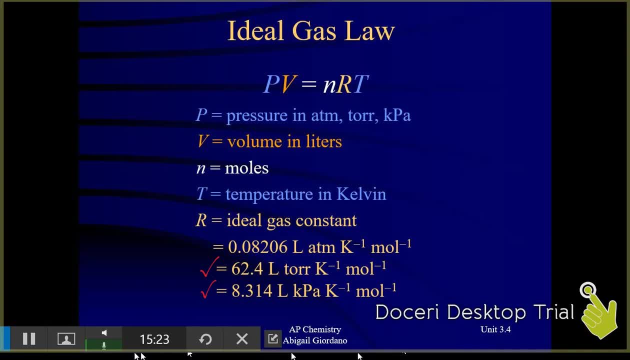 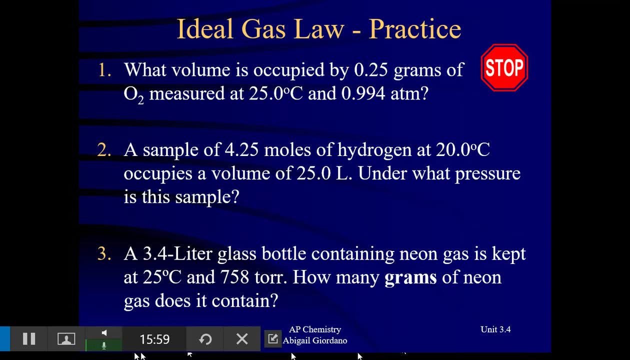 If my pressure's in kilopascals, I'm gonna use the third one, okay. So what I would like to do is just a quick practice with you. Okay, These are just three quick little ideal gas law problems to kind of get your brain back in gear. 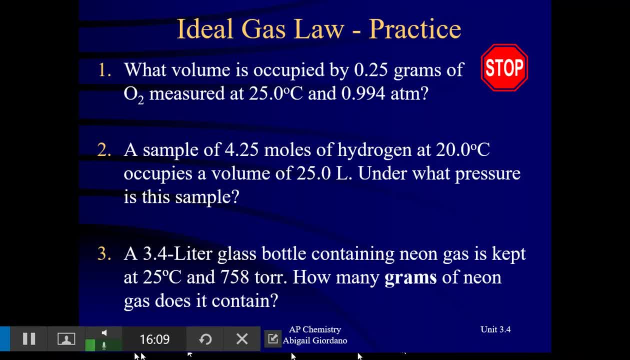 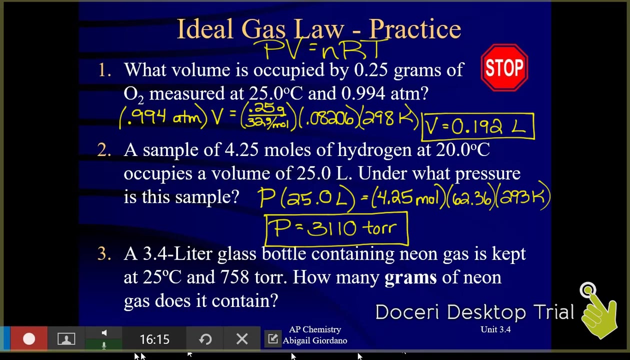 remembering how to use the ideal gas law. So pause your video and try these problems. All right, let's see how you did. Let's check your answers. So I was only able to fit the answers for one and two on this slide. 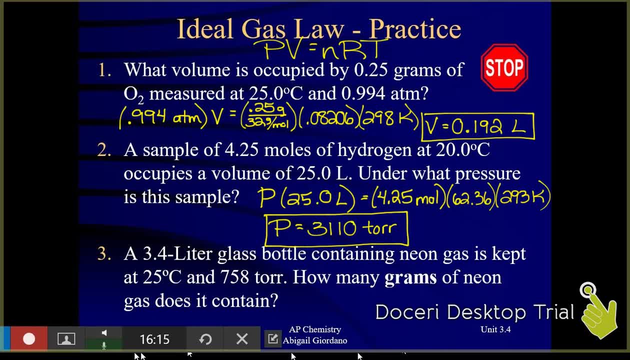 but I'll show you the answer to number three in just a second. So one and two, both are pretty straightforward. The only thing that's a little pinky about number two is just that pressure being the unknown, you get to choose what units. your final answer is in: 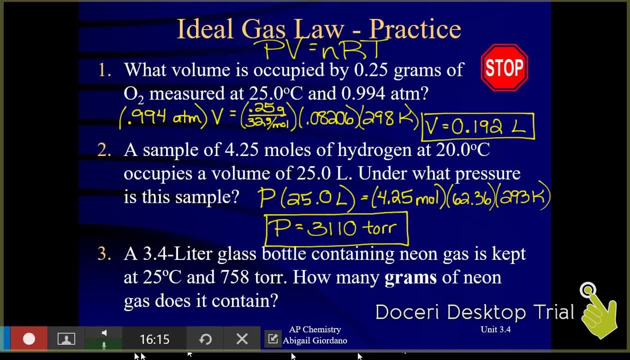 I chose to use the ideal gas, constant 32.5.. Okay, So I chose to use the ideal gas, constant 32.36, and thus my answer comes out in units of torr. I could also write it in millimeters of mercury. 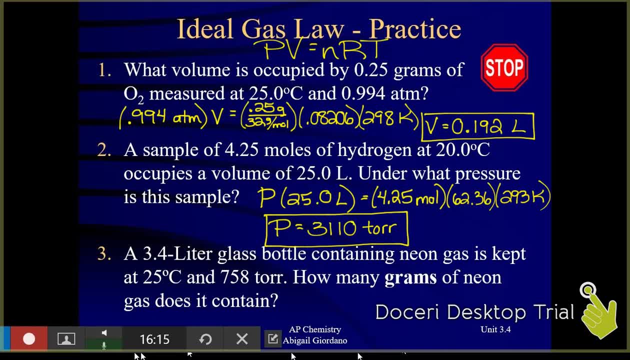 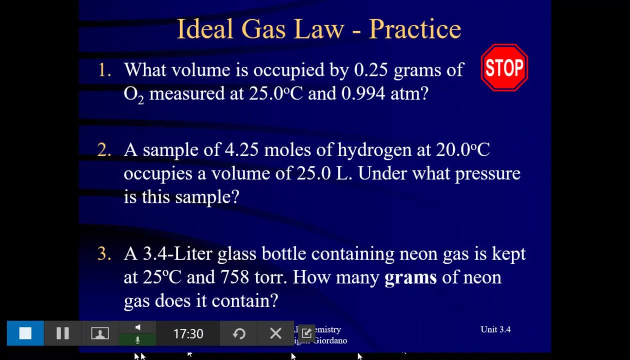 If you chose a different value for r, like 0.08206,, you're gonna get a different number and your answer will be in atmospheres. Okay, let me show you the answer for number three. Let me pull that up for you. 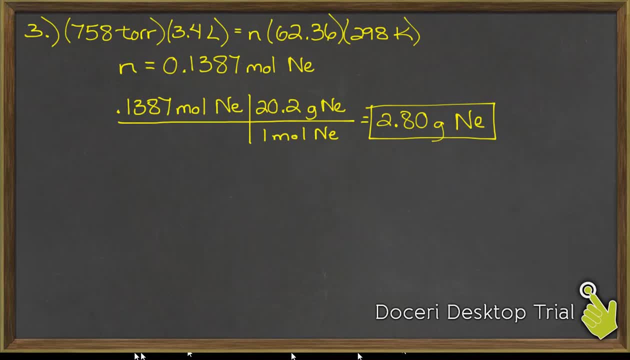 So number three asks you to solve for the mass of the gas. but mass is not one of our variables in the ideal gas law, So you had to solve for moles first and then convert it to grams. So that was just a little bit of a warmup. 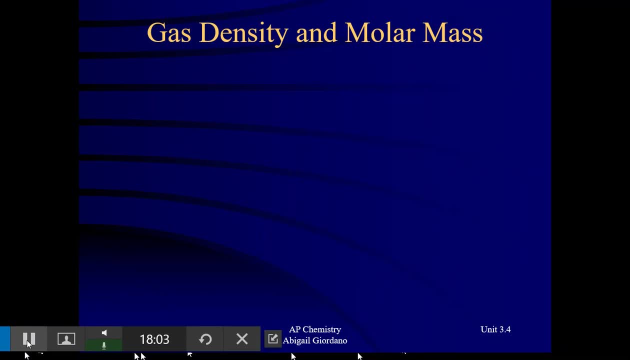 So one of the applications that you could use for this was- What was the application of the mass of the gas? Okay, so one of the applications that you could use for this that you can do with the ideal gas law, you can relate it to density and molar mass. okay, 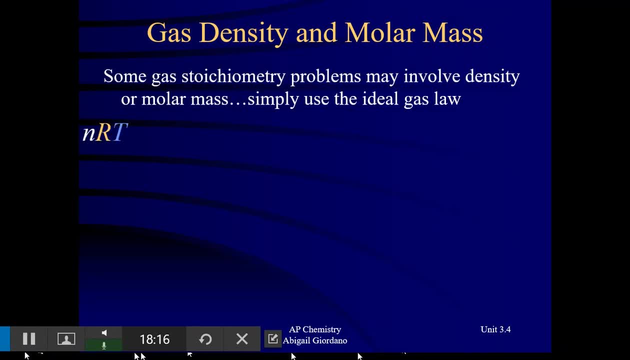 Now I realize that neither one of those things is in the ideal gas law. There is not a variable for density, there is not a variable for molar mass. but they're in there, they're just hidden. Okay. so here's the thing. 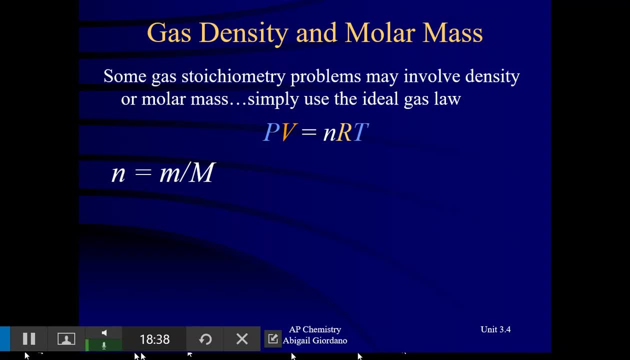 All right, go with me on this. Lowercase n means moles of gas, right, Right, okay, You all should agree that you can always solve for moles by dividing mass by the molar mass. So this little m here is the mass of the sample. 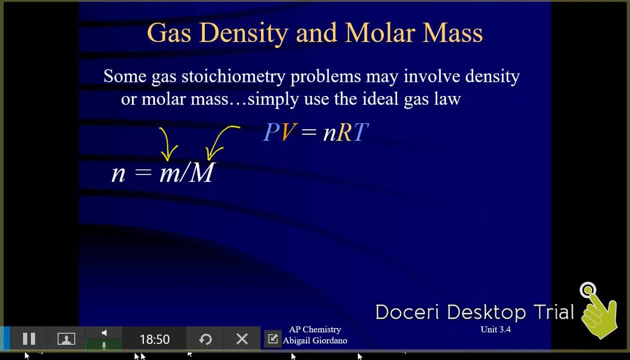 and this capital M is molar mass, off the periodic table. So think about it: Grams divided by molar mass will always give you moles. Okay, fine, Let's take that and substitute it in to the ideal gas law. Okay, all I've done is just substitute that in. 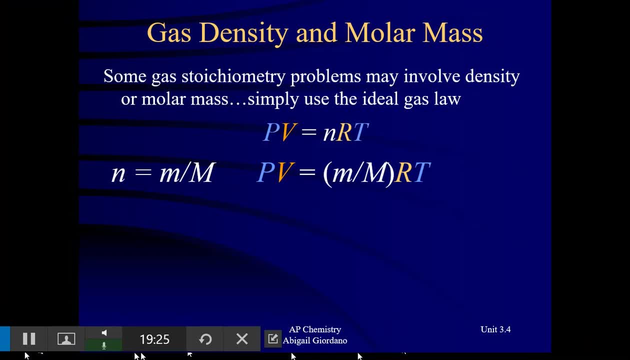 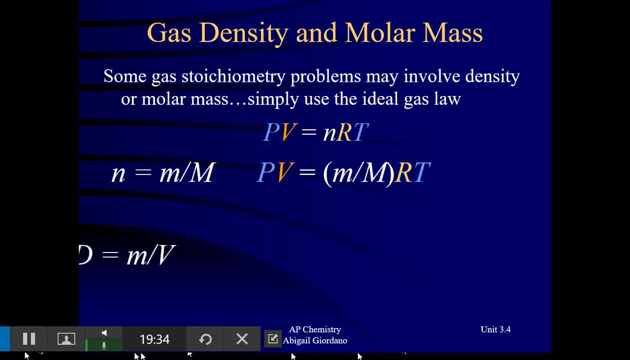 To isolate density. Okay, remember back from eighth grade: density is mass divided by volume. Well, look, I've got mass, I've got volume. I could rearrange that equation and isolate density on one side. okay, And I've got this little memory trick here, okay, 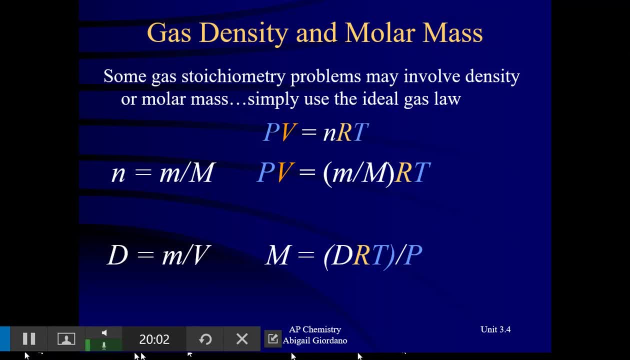 And I've got this little memory trick here. okay, This is not on your equation sheet. okay, But if this capital M, that's molar mass, this is density. okay, This is an equation you are always welcome to use, okay. 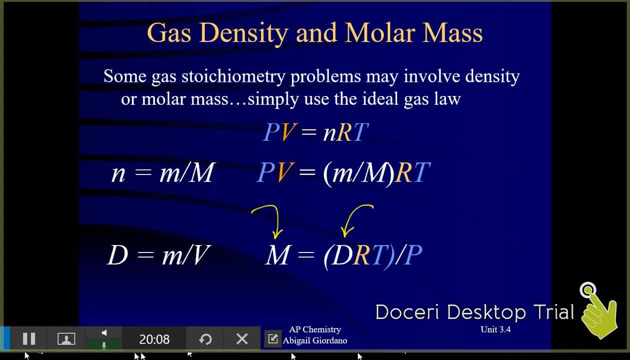 Molar mass equals density times the gas constant, okay, Constant times. temperature over pressure. M equals dirty P, Eww, gross dirty P, yuck, I'm a child. Anyway, if you ever have a gas law problem where molar mass is involved, 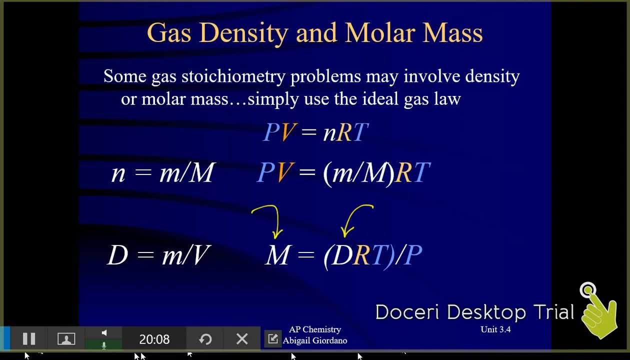 or maybe they don't tell you what gas it is and you have to figure it out. solving for the molar mass would be one way to solve it. One way to do that, okay. Or if a problem involves density, you can always use this equation. 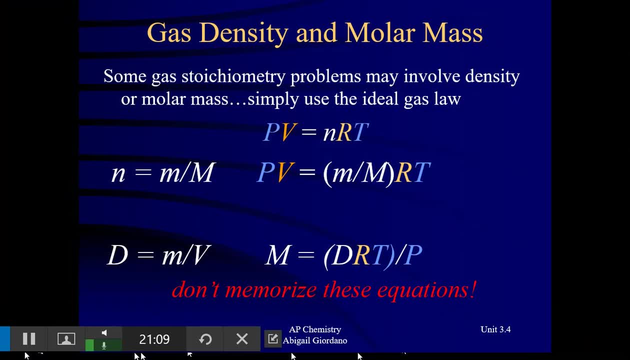 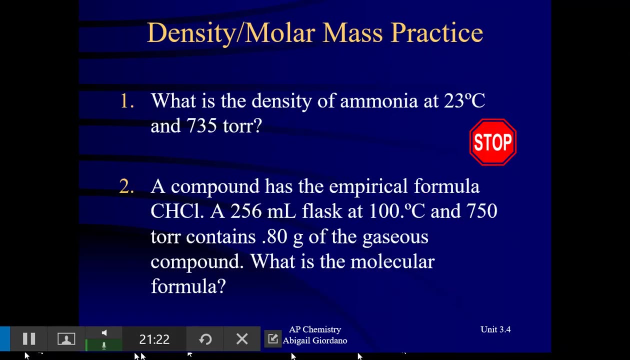 So I say: don't memorize, because you can always rearrange the mathematical expressions to isolate density on one side, But if you want to memorize it, who am I to stop you? All right, so what I want you to do. 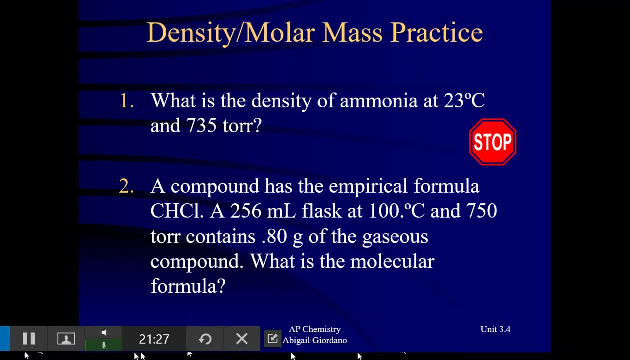 these are some practice problems that involve density, That involve density and molar mass. So I want you to pause your video and give them a try. All right, so let's check your answers, Let's see how you did. Sorry if it's a little messy. 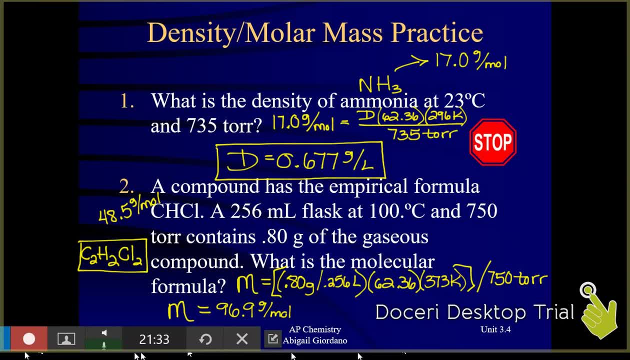 So, in number one, you had to know what the formula for ammonia is And, ladies and gentlemen, you should. Ammonia is NH3, and the reason I say you needed to know the formula is because, in order to use dirty pee, 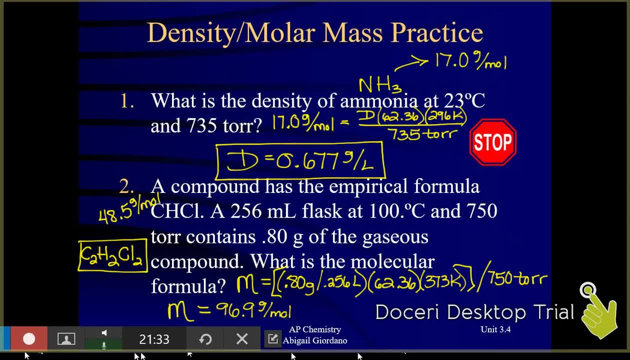 you had to know its molar mass. okay, I solved for the density in number one. How did I know that the units were gonna be grams per liter? Well, I knew it would be grams per liter because, remember, dirty pee came from. 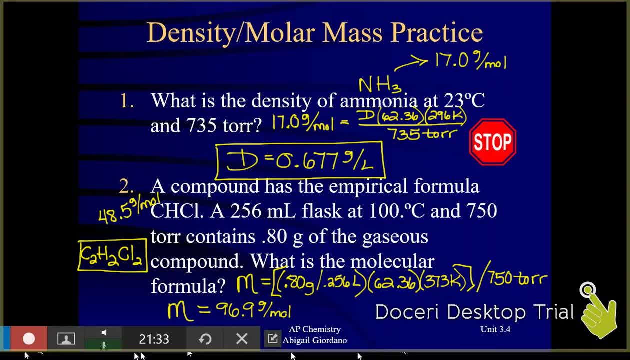 the ideal gas law and the ideal gas law, you have to have your volumes in liters. Now, in number two, the only unknown was the molar mass of the gas, which I solved for right there. Okay, it is an empirical molecular question, all right. 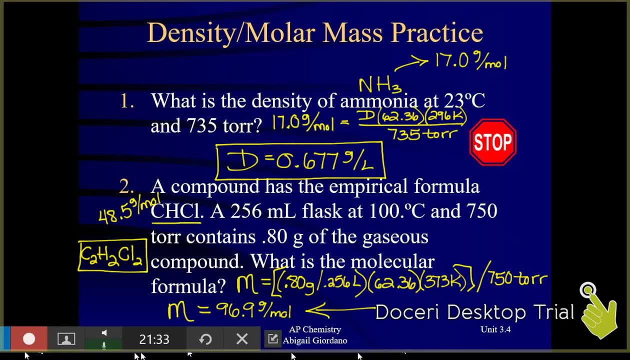 But they gave us the empirical formula, and there is its molar mass. Do you notice that the molar mass I solved for in number two is just about double that number? So here's my molecular formula: It's double all the subscripts. 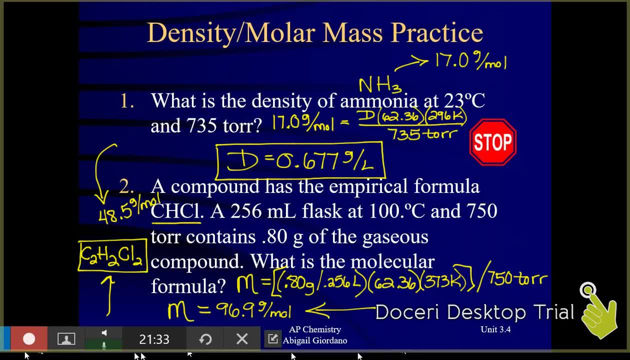 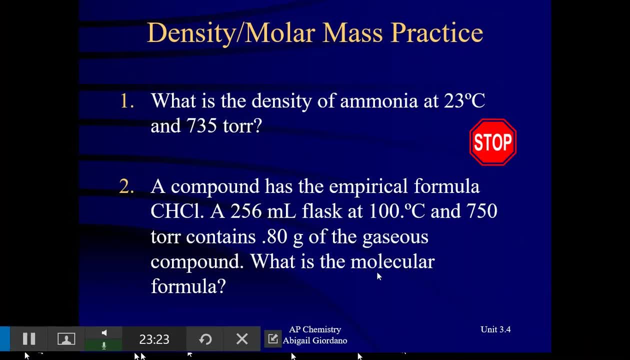 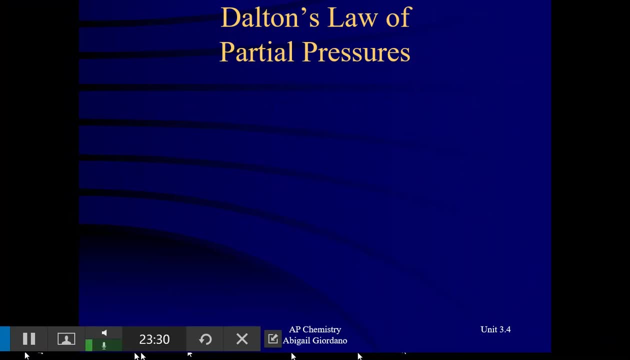 Okay. so sometimes they can link a gas law problem back to something that we did back in unit one. That happens, Be fair warned. Okay. now the last thing we're gonna look at, guys, is: what do you do when you have not just one gas? 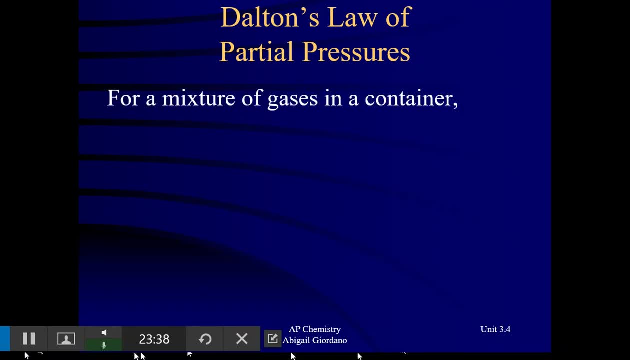 that you're dealing with, but multiple gases, Okay, a mixture of gases. Well, each gas is going to have its own what's called partial pressure, and that's what these variables- P1,, P2, P3, if there's three gases, it's gonna have its own partial pressure. 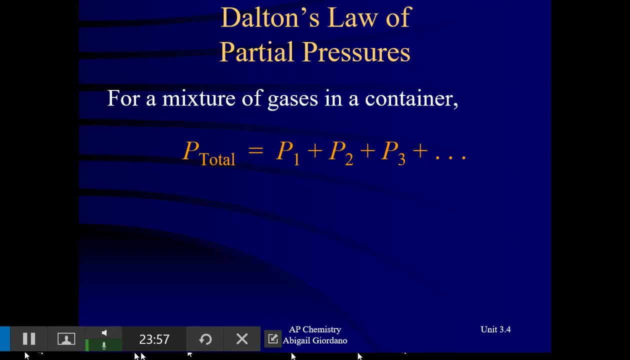 And that's what these variables- P1, P2, P3,. if there's three gases, each gas is gonna have its own partial pressure and you add them together and that will be the total pressure, And it doesn't have to be three gases. 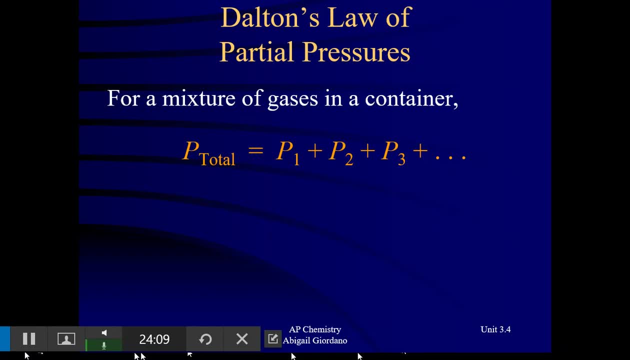 It can be any number of gases. So that's an equation that you'll use sometimes. Here's another one that you'll use. Okay, now let me make sure you understand what these variables are. okay, This is, of course, what it is above. 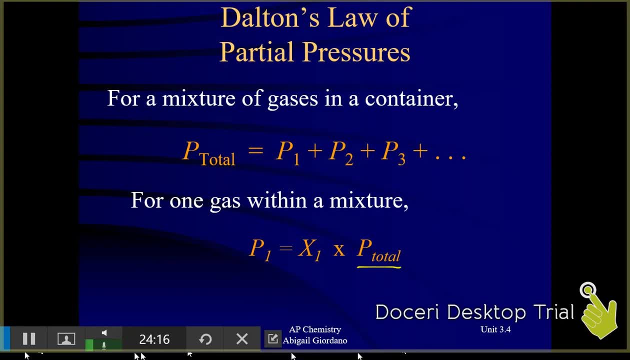 This is the total pressure within this mixture of gases, all of them added together, This one P1, that would be, if we're zeroing in on one of those gases within the mixture, P1 would be the partial pressure of that one gas. 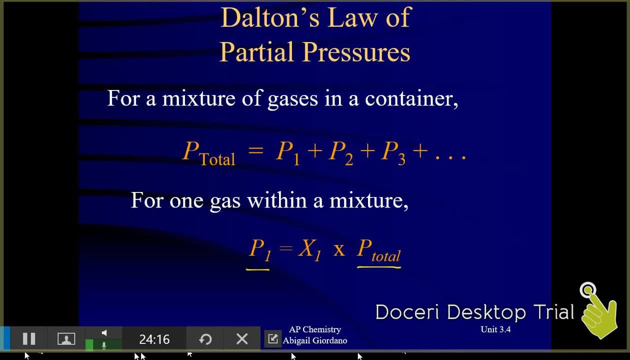 that we're focusing our attention on. This guy X1, is something called P2.. This guy X3, is something called the mole fraction, And both of these equations are on your equation sheet and the mole fraction is actually defined for you. 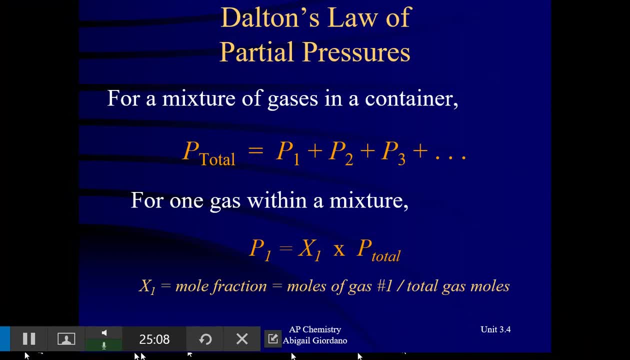 on your equation sheet. It tells you how to calculate it. Whatever this one gas is we're focusing our attention on, we're gonna look at how many moles of that gas are there and divide by the total moles of gas in the entire equation. 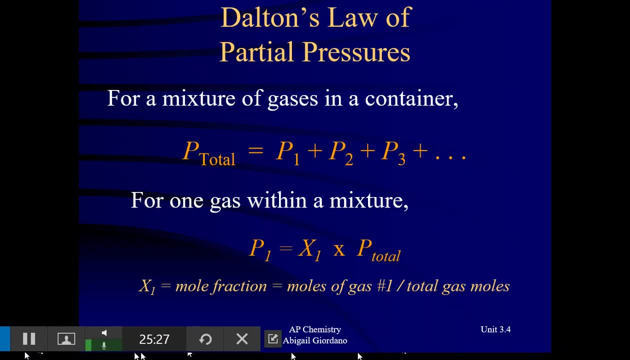 So this is the mole fraction. It's the mole fraction of the entire sample. It's kind of like a percentage, except we don't multiply by 100, okay. And mole fraction, since it's moles divided by moles. 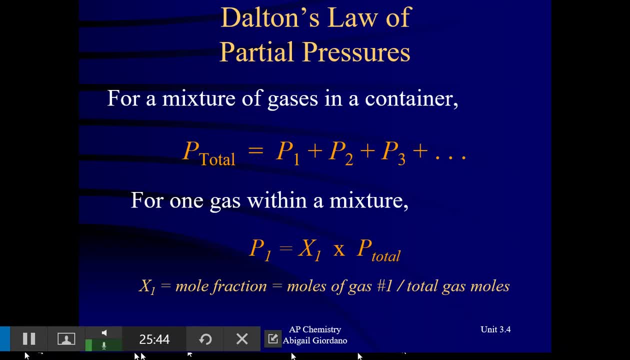 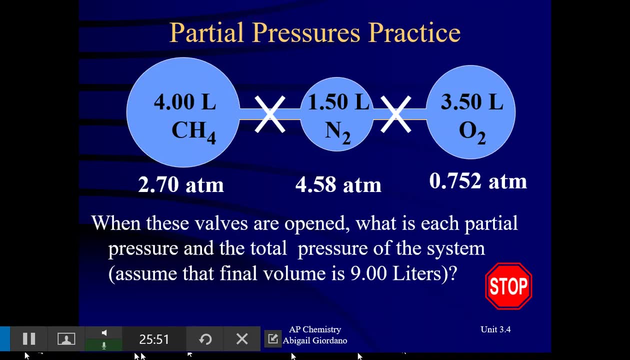 and those units cancel out. mole fraction is a unitless entity. Okay, so these are two equations that you might use when you're dealing with multiple gases all mixed together. This is a classic partial pressures question. I'm gonna set the scene for you. 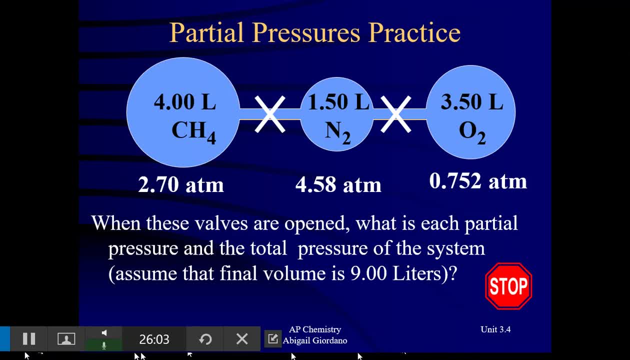 and then I want you to try it and see if you can figure it out, This diagram that you're looking at. there are three separate gases. Those Xs represent valves And right now the valves are closed. The gases are not mixing. 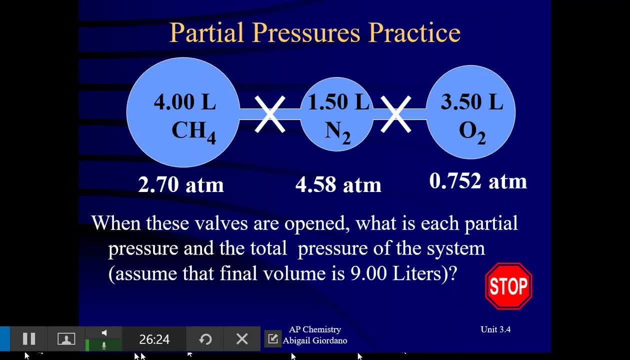 Each gas has its own individual volume. Each gas has its own individual volume. Each gas has its own individual pressure. When the valves are opened. okay, now stop there. Think about what's going to happen. Remember what we said: gases mix spontaneously. 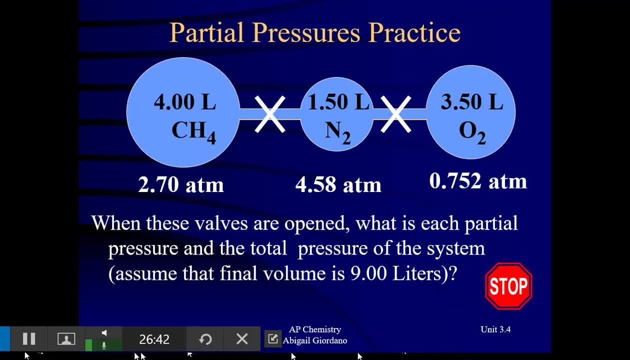 And what else did? we say Gases will fill the entire space that you give them. So all three of those gases are gonna spread out and fill that entire space And they're all gonna mix together. So when that happens, I want you to solve for the partial pressure of each gas. 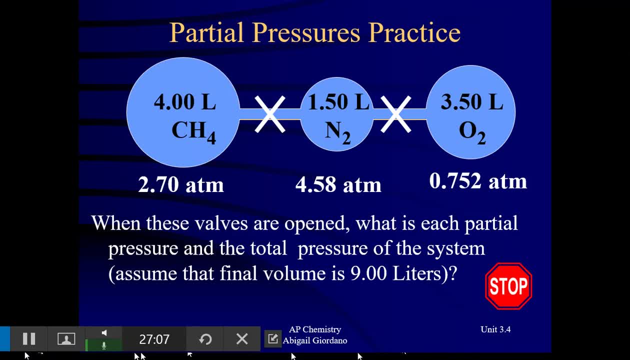 and then tell me what the total pressure is. And I'm gonna leave you with a hint before you pause your video and try it. Here's the hint: You have to use Boyle's law to solve this problem. Try it. All right, let's see how you did. 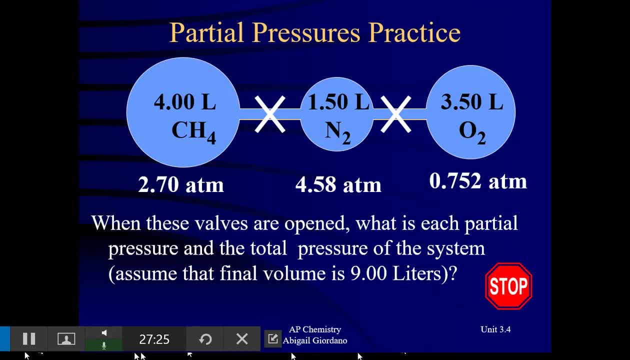 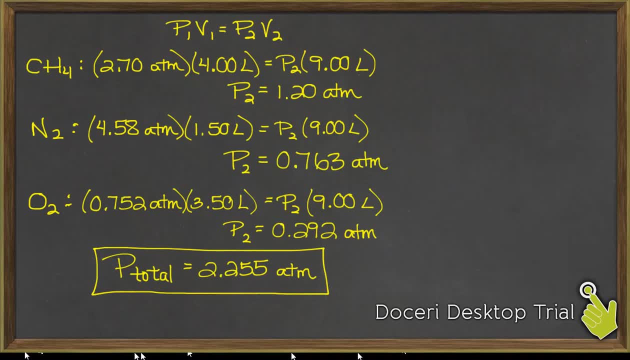 Remember? the hint was: you have to use the pressure, You have to use Boyle's law. So this is what I did For each gas individually: I used Boyle's law to solve for the new pressure. Okay, now just look at the first one: methane, for example. 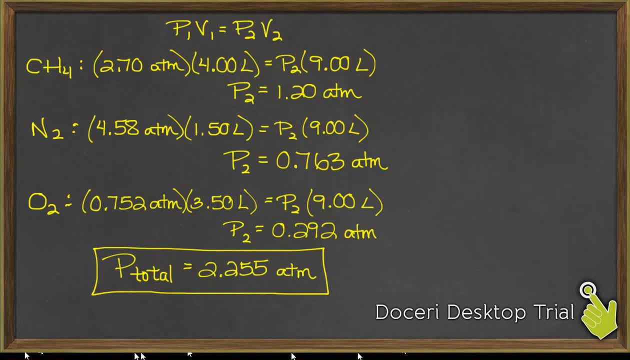 Okay, it's pressure was 2.7 atmospheres, but then we let it roam free and we let it spread out, Okay, And then we put it into the whole space. Think about Boyle's law: If we increase the volume, the pressure should go down. 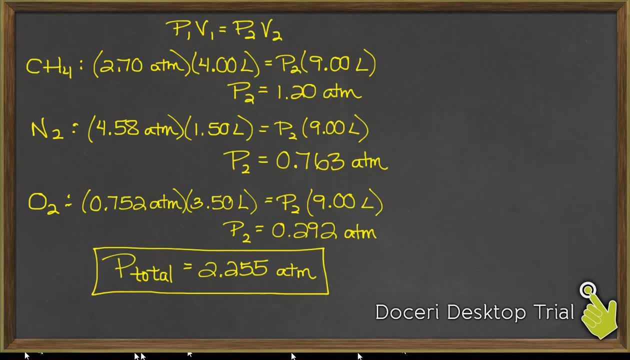 And it did Look at the new pressure for methane: 1.20 atmospheres. It did decrease, So did nitrogen, so did oxygen. How did I get that total pressure? I added all of the individual partial pressures together. Okay, this is a classic AP Chem kind of question. 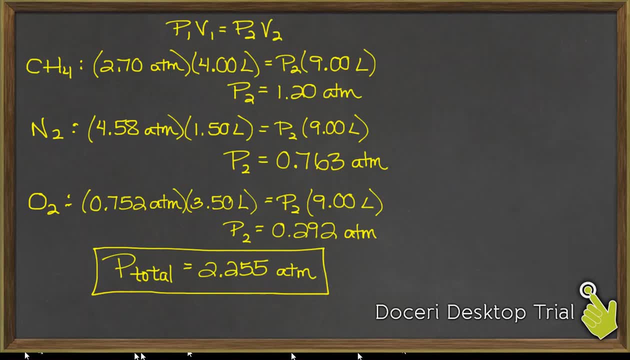 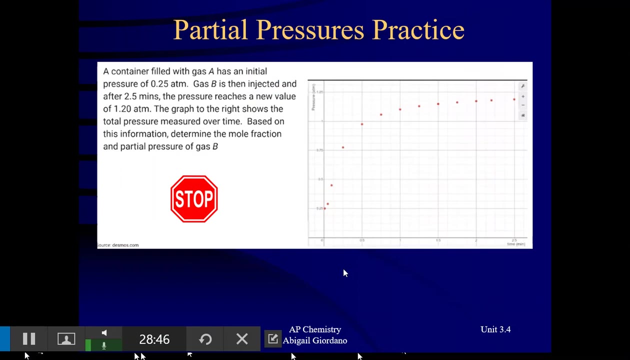 They love these questions with the container, with the valves, and they're closed at first and then they open them. They love questions like that. okay, All right, let's look at one more. okay, And I stole this from one of the AP Daily videos: okay, 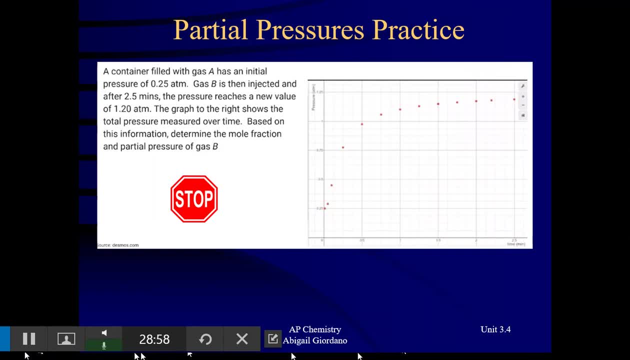 But it's still a partial pressure problem. all right, It says a container filled with gas A has an initial pressure of 0.25.. Okay, fine. Gas B is then injected and after two and a half minutes the pressure reaches a new value of 1.2 atmospheres. 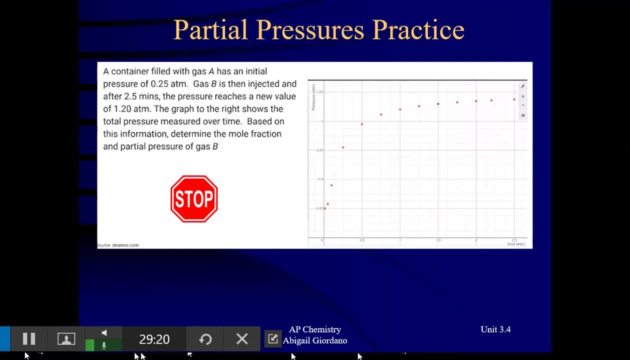 Okay, stop there. Notice the pressure went up? Well, it should, because we stuffed more gas in there, right? Aren't there going to be more collisions because there's more stuff in there, Okay. the graph to the right shows the total pressure measured over time. 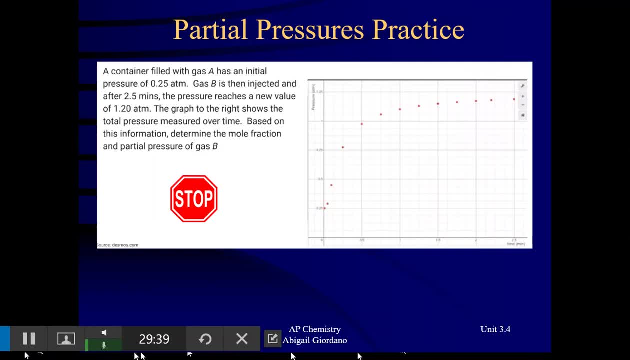 Based on this information, determine the mole fraction and partial pressure of gas B. okay, So if you want to pause the video, see if you can figure it out. I'm going to go through it and talk it out with you. All right, let's talk this out a little bit. 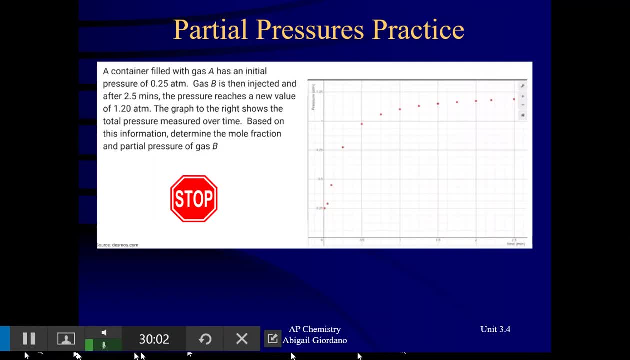 First of all, guys, the graph there is almost just sort of a distractor. You really don't need that graph. okay, Let's focus on solving for the partial pressure of gas B first. okay, We know, We know what the pressure of just A was.